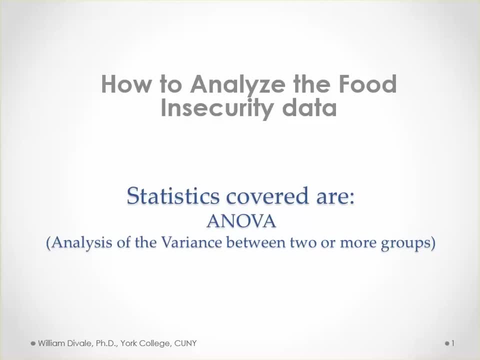 Okay, folks, this is Dr DiValli, and this is the third video in the series How to Analyze the Food Insecurity Data, And the statistics covered in this video are the ANOVA, which stands for the Analysis of Variance Between Two or More Groups, In other words, 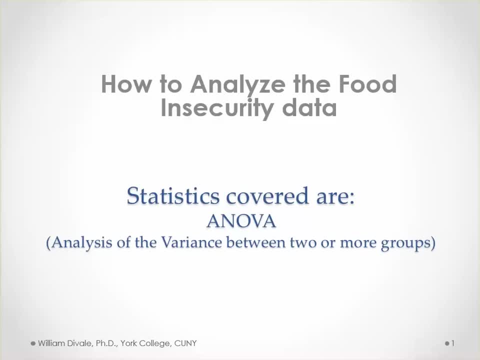 the ANOVA statistic analyzes the average scores and the variation within those scores between two, three or more groups and tells you if the differences between them are likely just to be due by chance or perhaps are due to some other theoretical factors that are causing it. 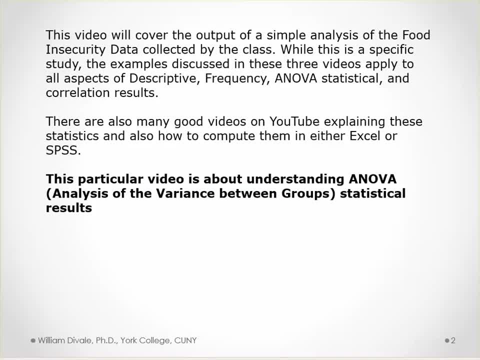 Now again. this video will cover the output of a simple, simple analysis of the food insecurity data collected by the class. While this is a specific study, the examples discussed in these three videos apply to all aspects of descriptive frequency, ANOVA, statistical and correlation results data. There are also a good many 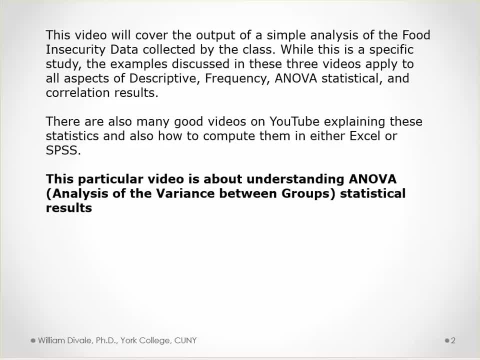 videos on YouTube explaining these statistics and also how to compute them using either Excel or Excel. These are the examples of how to use ANOVA statistical analysis and the ANOVA statistical analysis. This particular video is about understanding ANOVA analysis of the variance between groups. 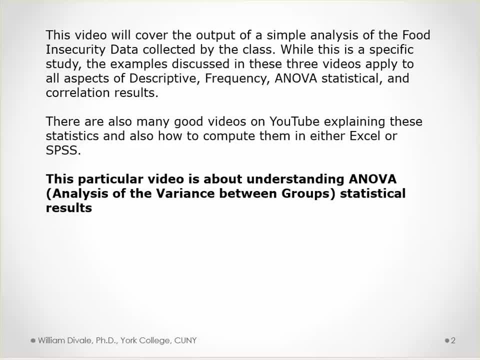 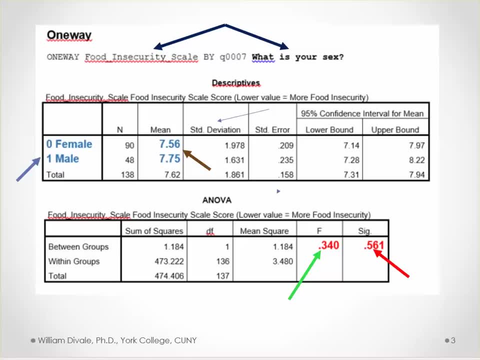 statistical results. In other words, it's not about calculating it, but it's about understanding the results when you get them. Now in this slide, I'm showing a typical output of an ANOVA statistic, which you also have to know. 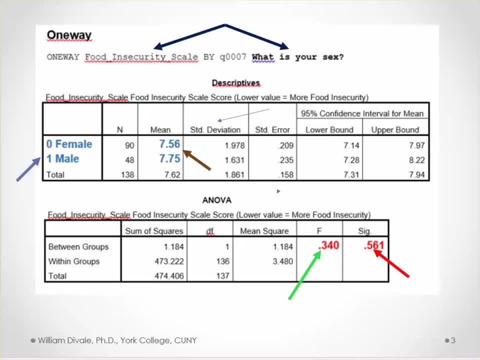 Which also includes the descriptive statistics, which I think helps to understand and interpret what's going on. So these arrows point to the aspects of the chart that I think are more important to focus on. So first, on the top, the two very dark blue arrows point to the two variables. on the study, 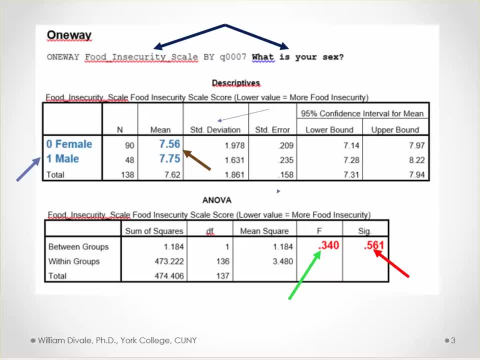 The independent variable, you might say, is general. The independent variable, you might say, is general. The dependent variable, you might say, is gender. What is your sex? And the dependent variable is the food insecurity scale score. In other words, we're looking to see if gender influences what a person's food insecurity 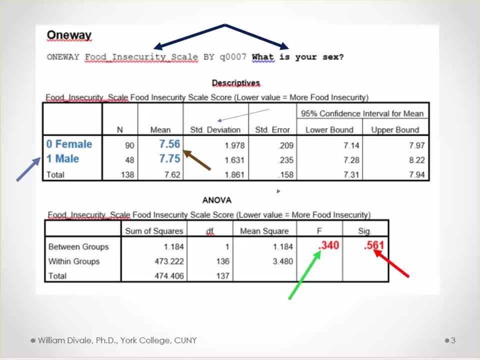 scale score would be. So if we look at the blue arrow on the left, we see we're comparing two groups, females and males, And the brown arrow showing the column of the mean scores. That means the average scores. For females, the average food insecurity scale score was 7.56.. 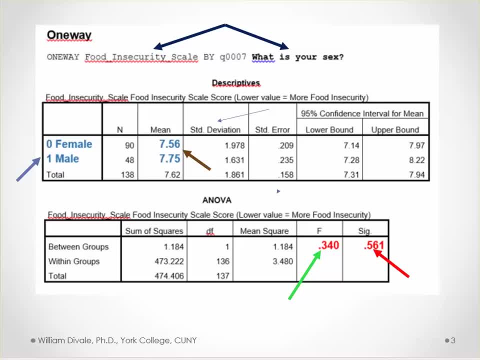 And for males it was 7.75.. So here females expressed more food insecurity than do males, Although the scores are in the middle range. In other words, these are scales of above 7.56.. And for males it was 7.75. 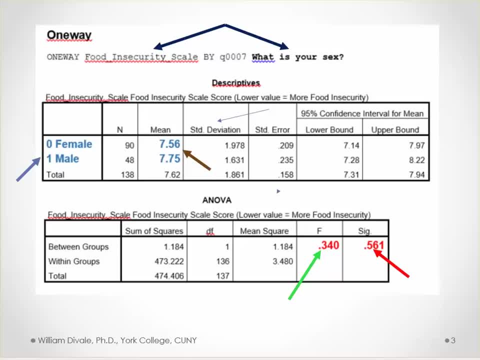 So here, females expressed more food insecurity than do males, Although the scores are in the middle range. In other words, these are scales of above 7.56.. They're not this. either group is not endangered just because of their gender. 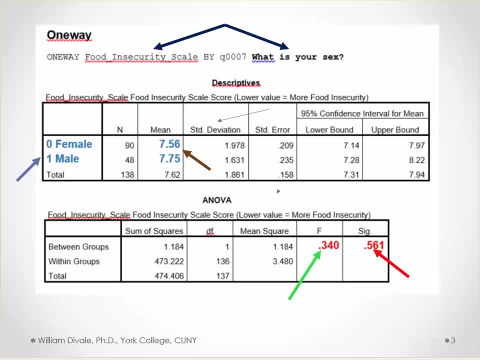 And the small blue arrow refers to the standard deviation, which gives you an idea of what the average amount of variation in scores are within each subsample. Now the lower chart shows the ANOVA results. okay, and what I need for you to focus on. 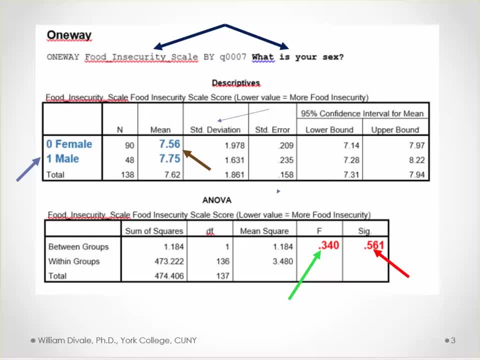 are. there's the F-scope score, which is the ANOVA F statistic, and that's a number. In this case it's 0.340.. And then the red arrow points to the significance level. That's the probability level. 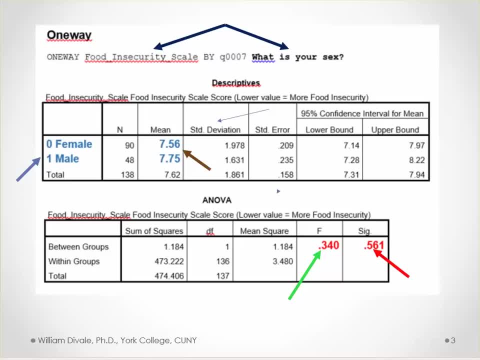 The higher the F score gets, the lower will be the significance score value. In this case, the significance score is 0.561.. So in other words that even though we find a difference between men and women in their hunger and security, this difference we found would happen. 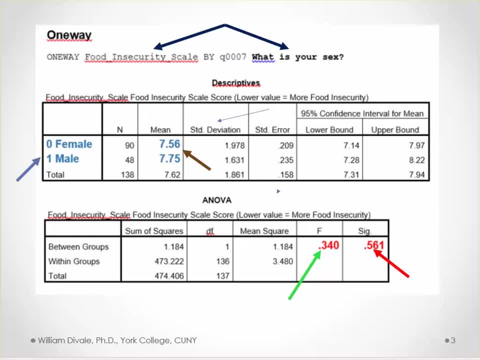 56% of the time. In other words, it's probably just due to sampling error of the particular sample of 138 people that we had here. So the difference is not statistically significant. For it to be statistically significant, that number on the SIG would have to be 0.05 or 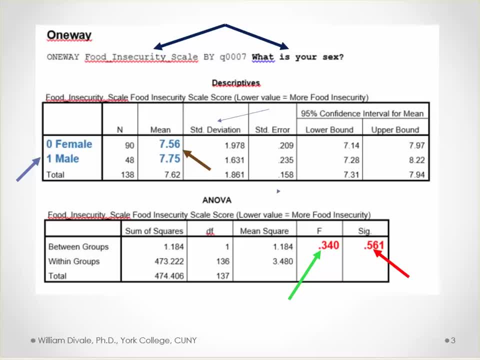 smaller: 0.0499, 0.049, 0.04, or 0.05.. But anything higher than, say, 0.0501, that would be above the cutoff point that scientists use To say the results are likely to be just due to chance sampling errors and not to any. 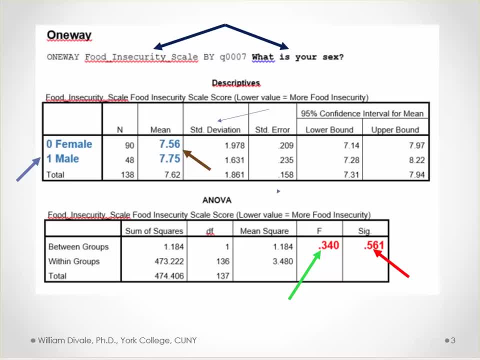 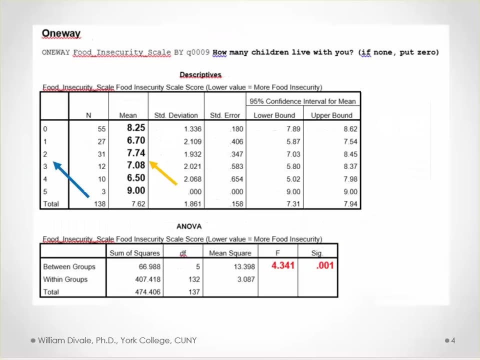 kind of influences of one variable upon the other. This is a conservative interpretation, but this is the way we make fewer mistakes. Now, this is the difference on food insecurity scale by sex. So let's look at the next one, which is how many children 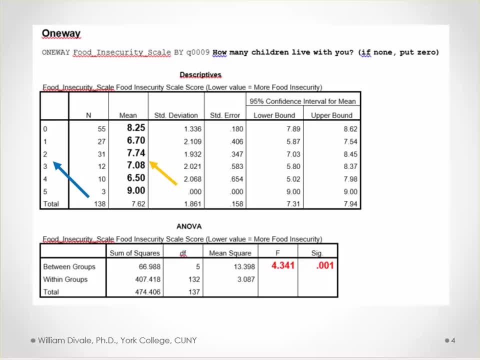 How many children live with you. So if we look at the blue arrow, that points to the number of children that's been reported: 0,, 1, up to 5.. The orange arrow is the average food insecurity score of those people. For example, 55 people. 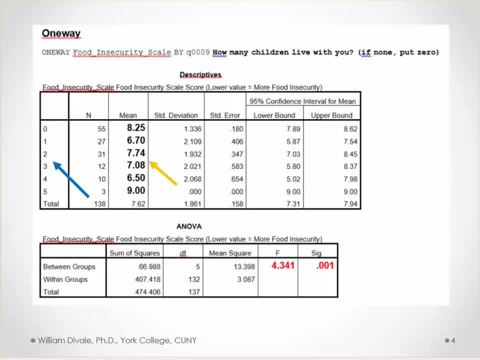 in the sample said they did not live with children and their food insecurity score was 8.25.. And if you look, there's only two which show low numbers: The one living with one child, there's a 6.7.. And also living with four children, there's a 6.5.. But someone has 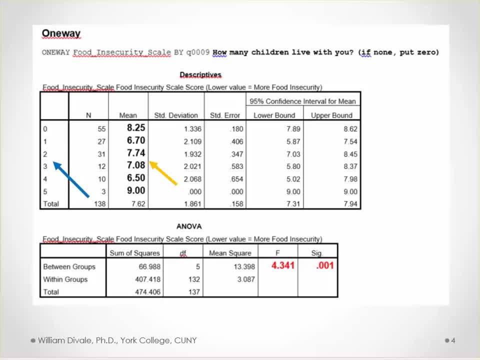 five children and their score is 9.. So they're not experiencing any food insecurity. Now let's look at the bottom chart And here the F-score now is 4.341.. It's much higher And the significance level is 0.001.. That's much smaller than the F-score And the F-score. 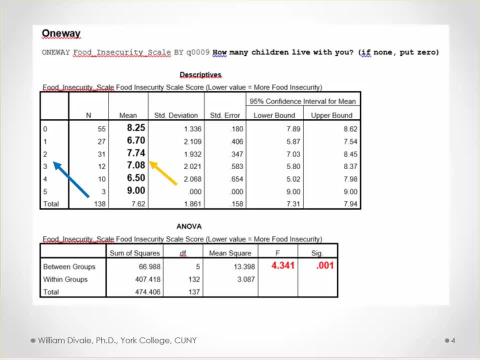 is higher than 0.05.. So that's saying that the differences in these food insecurity scale scores by the number of children a person has. these differences would only occur by chance one out of a thousand times if we did this study. So that's telling us that the number of children you have living with you does influence your 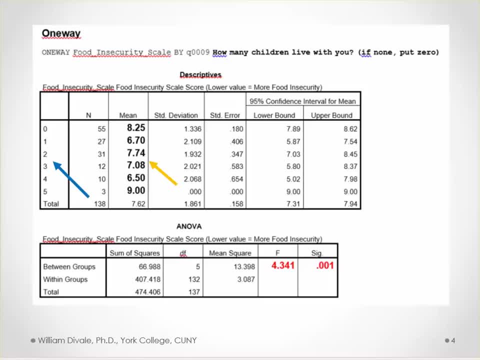 food insecurity scale score, And in particular, there are other factors, of course. I mean the person with four children has high food insecurity, But so does the 27 people who have one child. So it's not just the number of children alone, It's also other factors, probably related to income. 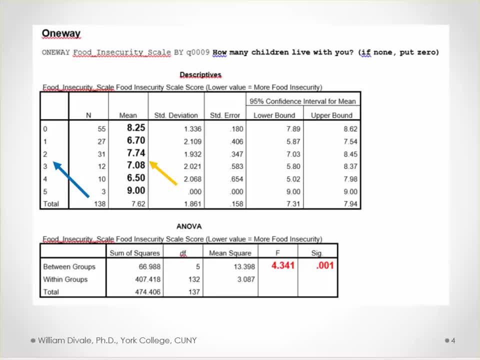 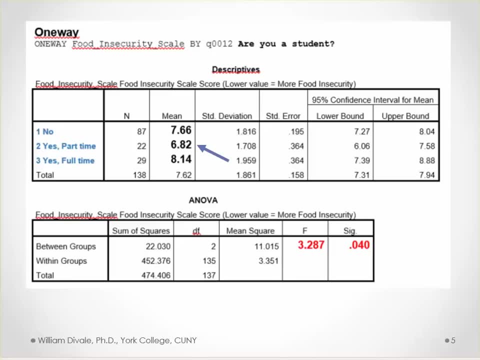 or whatever that hopefully our other slides will show us. And now here we have, an over between food insecurity score and if you have a KEE, the Un współ faire simply stands for fellow who have zero Among folks with food insecurity. 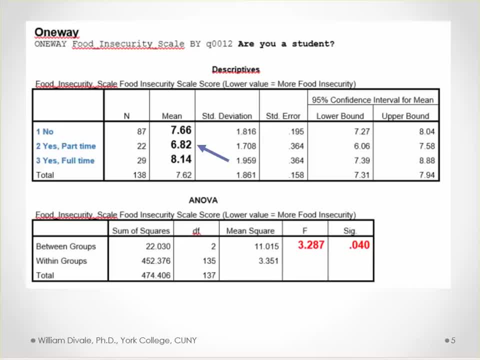 Now there were three answers to that question. No, you are not a student, Yes, a part-time student and yes, a full-time student. And if we look at the mean scores on the food insecurity scale, we see it's lowest for the part-time students. 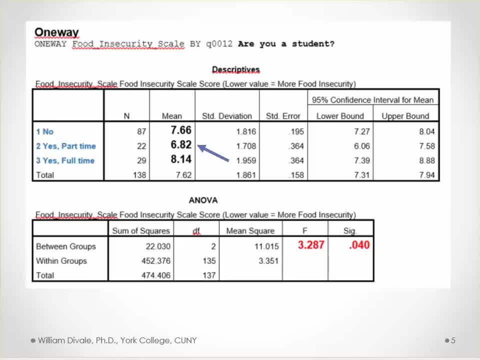 So the non-students either. maybe they worked and the full-time students had other means of support, So it's maybe the part-time student that had to work as well as go to school. their food insecurity scale scores were lower. 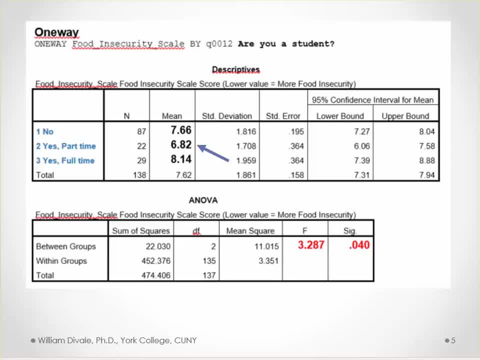 And again, if we look at the bottom, the F-score is 3.2, and the significance level is .04, which is smaller than .05.. So there's only a 4%. So there's only a 4% chance in 100 that these differences in food security scores could have happened by chance. 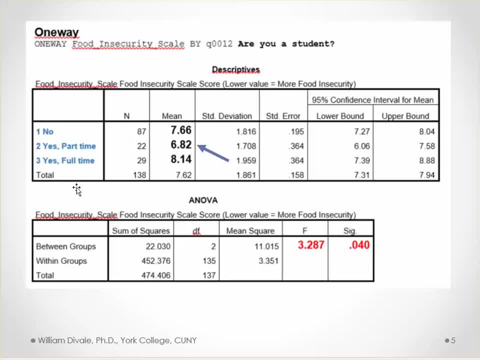 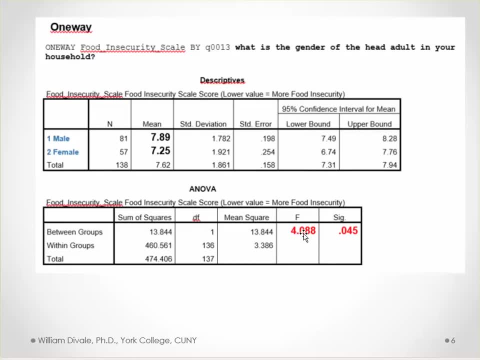 So, obviously, being a student and what kind of work you do influences your score. Okay. now what is the gender of the head of the household, the head adult in the household and their food insecurity? Okay, so if the gender was male, therefore, 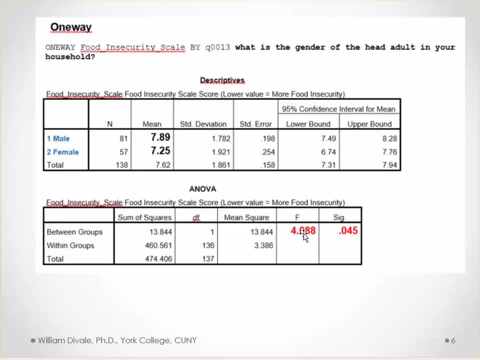 Okay. so if the gender was male, therefore, their food insecurity score was 7.89, but if it was female, their average score was 7.25.. And again, if we look, the F-score is 4.08, and the probability of that F being due to chance alone is .045,, which means it's only 4.5% out of 100.. 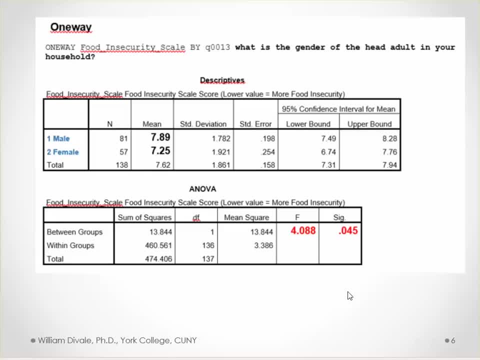 So it is below the 5% level of significance. So we would reject that. We would reject the null hypothesis that is due to chance and say that female head of households do experience more food insecurity than do male head of households. 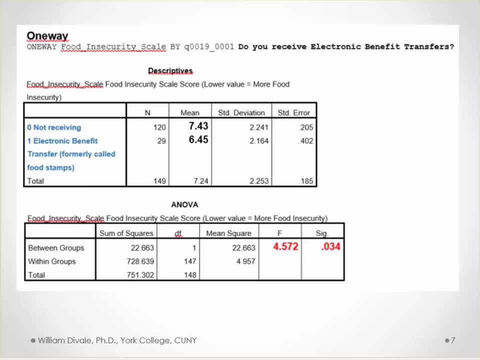 Now in this slide we're looking at, do you receive electronic benefit transfers? In other words, does the person receive food stamps And what is their food insecurity scale score? So if we look, We see that people who do not receive food stamps- that's the zero- their average food insecurity score was 7.43, while those who were receiving food stamps, their average score is lower, 7.45, indicating food insecurity. 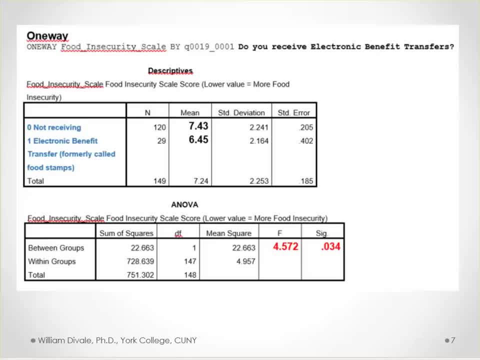 And if we look at the F-score again, it's 4.5, and the significance is .34.. So the likelihood that this difference Could have happened just by chance is less than 3.4% out of 100 times. we did this study. 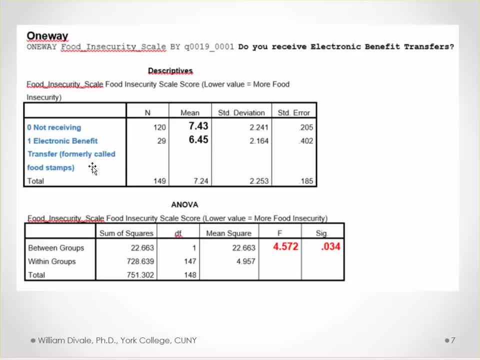 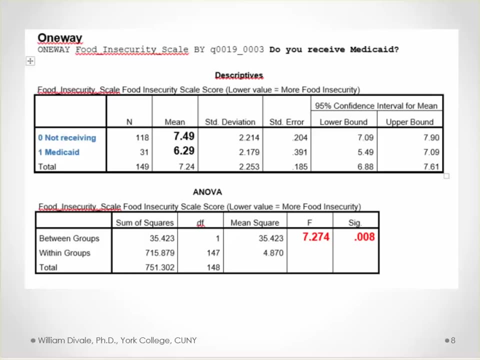 So people receiving food stamps do experience more food insecurity. In other words, they should be receiving food stamps. Now in this chart we're looking at, do they receive Medicaid And what is their food insecurity scale? And it's poorer people. 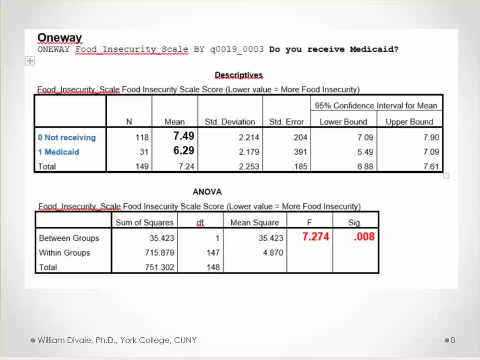 Do they receive Medicaid. So those not receiving Medicaid, their average food insecurity scale score is 7.49.. And those receiving Medicaid, it's 6.29.. And if we look this F-score on, that is 7.27.. 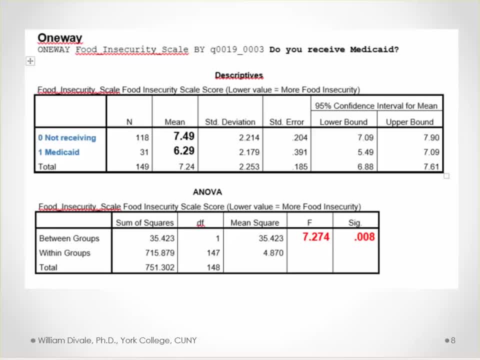 And the significance is .008.. In other words, that's less than If this study was done 1,000 times and only 8 of those times would we find differences In food insecurity this great or even greater, if there was truly no difference between people who received Medicaid or did not and food insecurity, so that people on Medicaid tend to be more insecure about food. 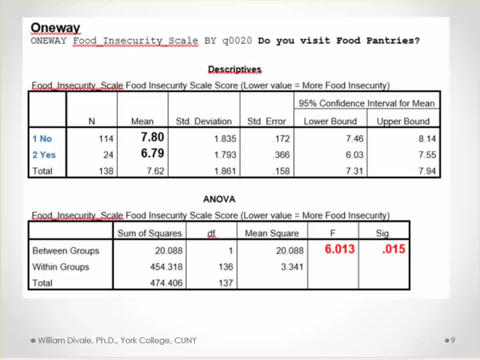 Now, finally, the last slide in this video is the food insecurity scale with. do you visit food pantries where you can get food for free? And if we again, if we look at the food insecurity scale, we'll see that there's no difference between people who receive Medicaid or did not and food insecurity.